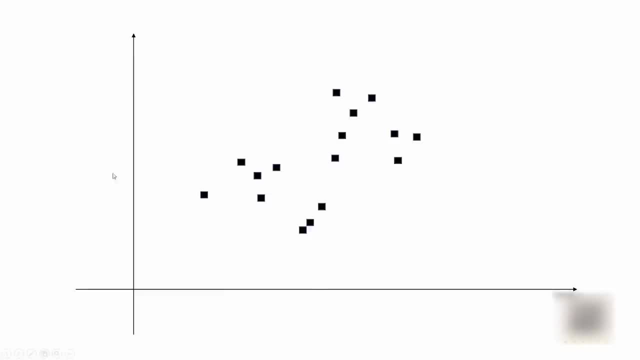 Let's say you have a data set like this, where x and y axis represent the two different features, and you want to identify clusters in this data set. Now, when the data set is given to you, you don't have any information on target variables, So you don't know what you are looking for. All you are trying to do is identify some structure into it, And one way of looking into this is these two clusters. Just by visual examination, we can say that this data set has these two clusters, And k-means helps you identify these clusters. Now, k in k-means is a free parameter. 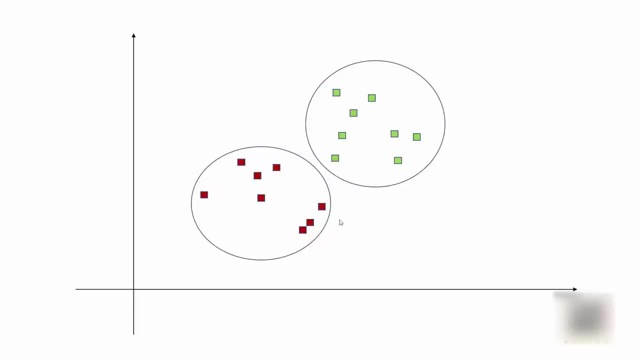 Before you start the algorithm, you have to tell the algorithm what is the value of k that you are looking for Here. k is equal to two. So let's say you have this data set. You start with k is equal to two And the first step is to identify: are two random points which you consider as the center of those two clusters. We call them centroids as well. So you just put two random points here. If your k was, 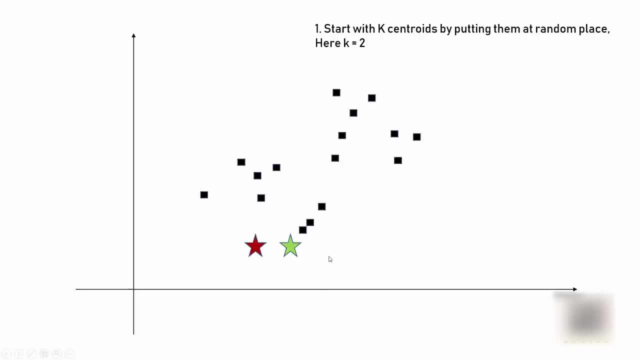 let's say three. then you will put three random points, okay, and these could be placed anywhere in this 2d place, doesn't matter. next step is to identify the distance of each of these data points from these centroids. so, for example, this data point is more near to this centroid, hence we'll say it belongs to red. 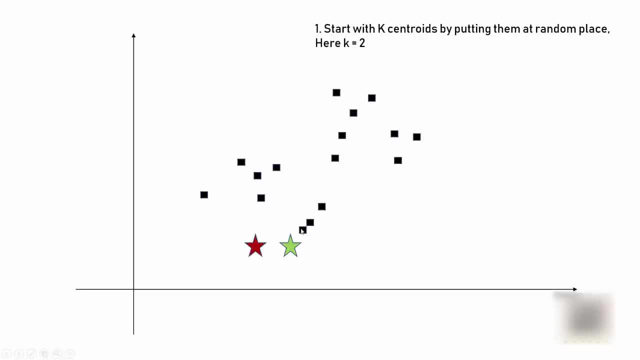 cluster, whereas this data point is more near to green, so we'll say this belongs to green cluster. the simple mathematical way to identify the distance is to draw this kind of line connecting the line between the those two centroids, and then draw a perpendicular line anything on the left. 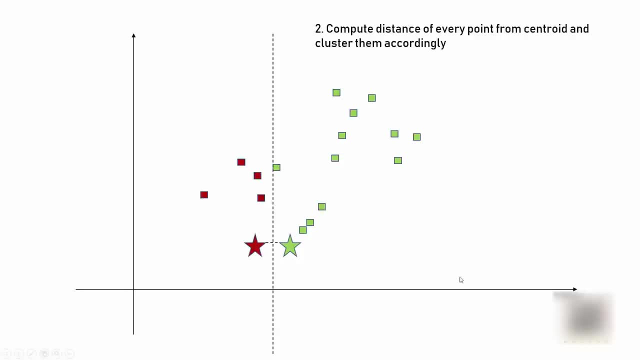 hand side is red cluster, on right hand side is green cluster. so there you go. you already have your two imperfect, clunky clusters, and now we try to improve these clusters. okay, so you started, you already got your two clusters. now we'll make them better and better at every stage, and the way you do that is: you will try to. 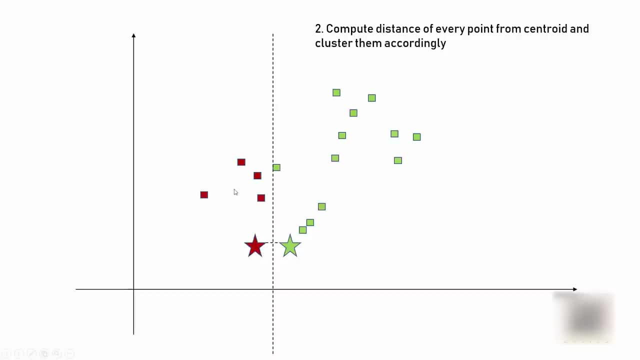 adjust the centroid centroids for these two clusters. for example, for this red cluster, which is these four data points, you will try to find the center of gravity almost, and you'll put the red centered there, and you do the same thing for green one. so you get this. 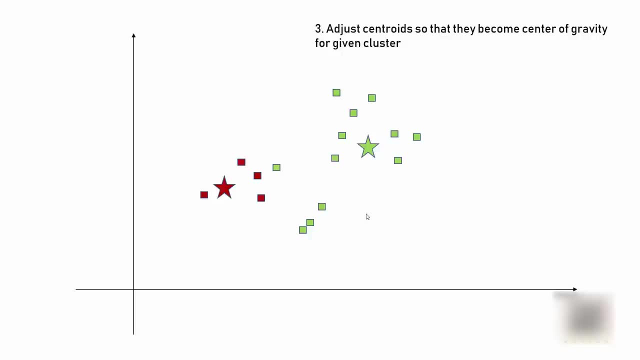 when you make the adjustment. and now you repeat the same process again. again, you recompute the distance of each of these points from these centroids and then, if the point is more near to red, you put it at them in a red cluster, otherwise you put it in a green, green cluster. okay, so you, you repeat the same method and see: 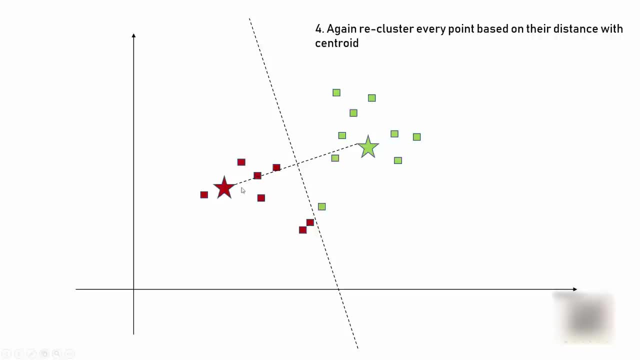 now these points got changed from green to red, so they're more near to red. that's why they are in red cluster. and you keep on repeating this process. you just recalculate your centroids, then recalculate the distance of individual data points from these centroids and readjust the clusters until the point. 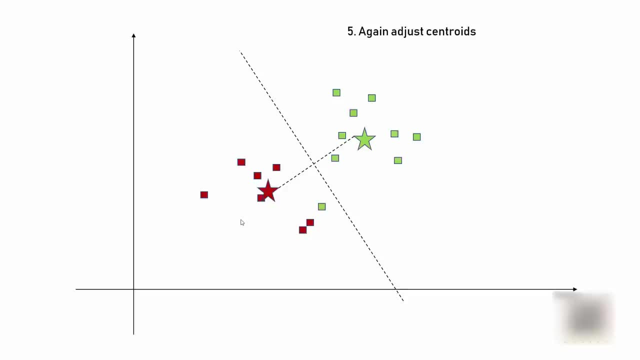 that none of the data points change the cluster. so here right now, see, there is only one green which is changing. it's a cluster, so now it's in red. but after this we are done. even if you you try to recompute everything, none of these data points will change their. 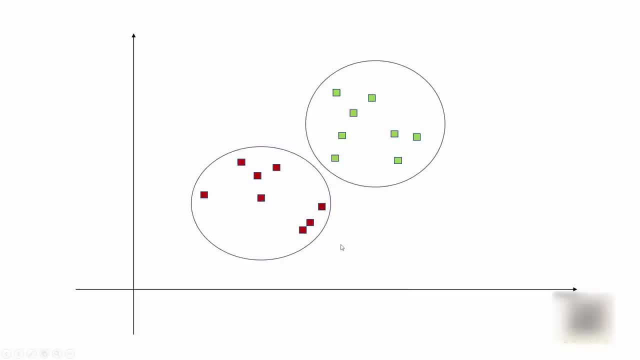 position. hence we can say that this is final. so these are now my final clusters. now, the most important point here is: you need to supply K to your algorithm. but what is a good number on K? because here we have two dimensional space. in reality, you will have so many features and it is hard to visualize that data on a scatter. 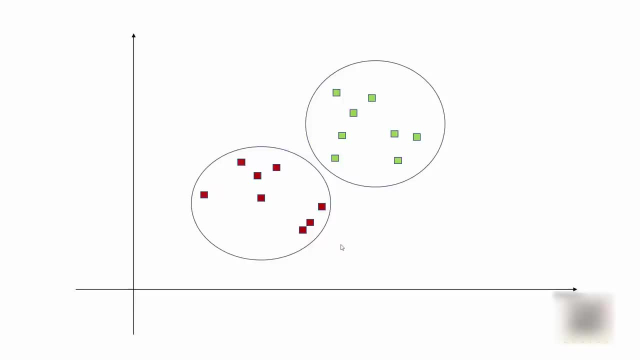 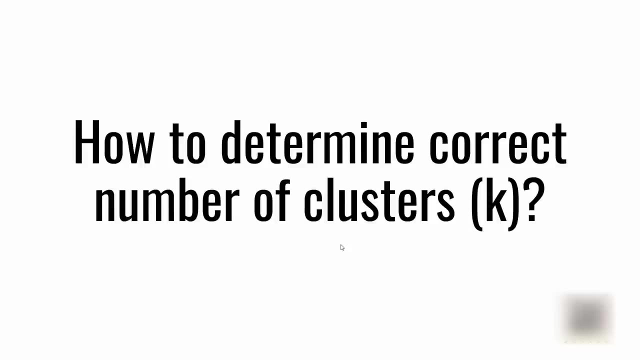 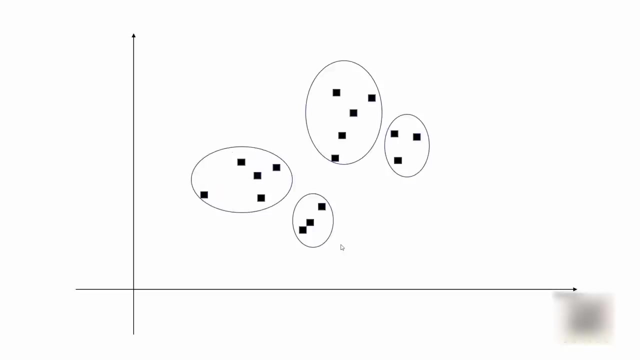 plot. so which case should you start with? well, there is a technique called elbow method. okay, and we'll look into it. but just to look at our data set, we started with two cluster, but someone might say, no, these are actually four cluster. third person might say, oh, they are actually six cluster. so you can see like different. 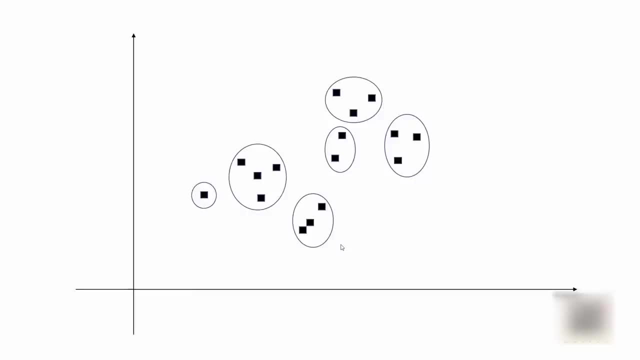 people might interpret these things in a different way, and your job is to find out the best possible K number. okay, and that technique is called elbow method, and the way that method works is you start with some K. okay, so let's say we start with K is equal to two and we try. 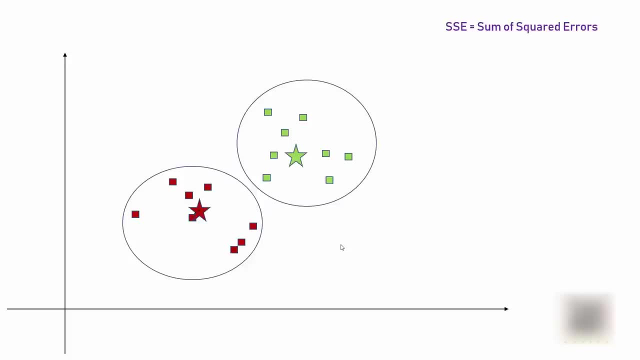 to compute sum of square error. what it means is, for each of the clusters, you try to compute the distance of individual data points from the centroid. you square it and then you sum it up. so for this cluster, we got sum of square error. so for this cluster, we got sum of square. 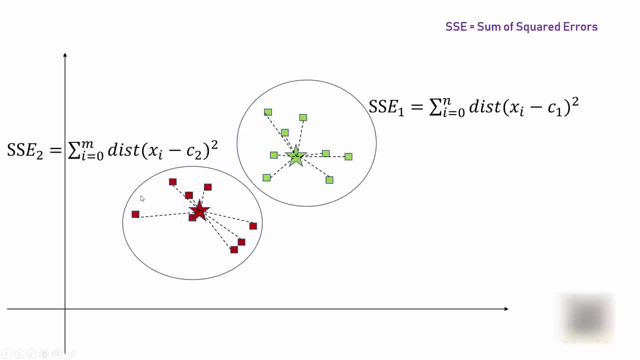 error one. similarly for the second cluster, you will get the error number two and you do that for all your cluster and in the end you get the total sum of squared errors. now we do square just to handle Negate value. there is nothing more than that. okay, so now. 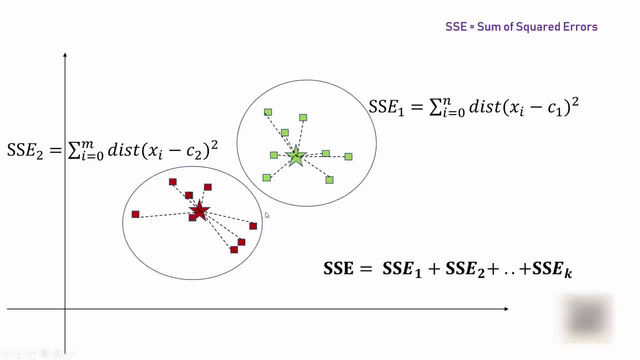 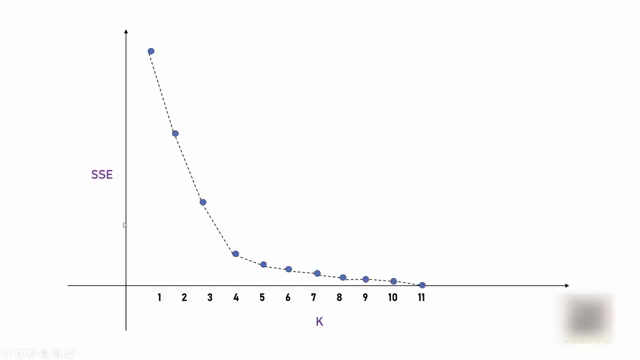 we computed SSE for K equal to two. you repeat the same process for K equal to three, four and so on. okay, and once you that number, you draw a plot like this: here I have K going from 1 to 11, and then on the y-axis I have sum of squared error. you will realize that as you. 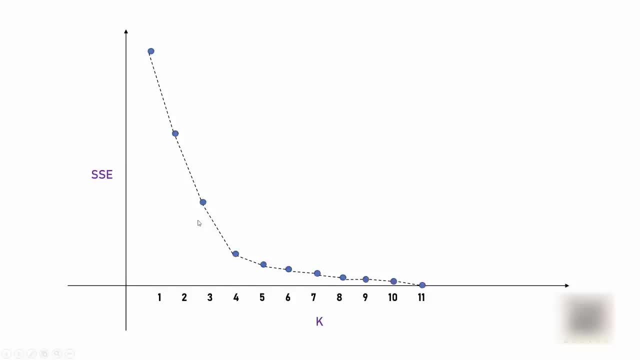 increase number of clusters, it will decrease the error. now it's kind of intuitive to think about it. at some point you can consider all your data points as one cluster individual, where your sum of squared error becomes almost 0. okay, so let's assume we have only 11 data points at 11 value of K, the 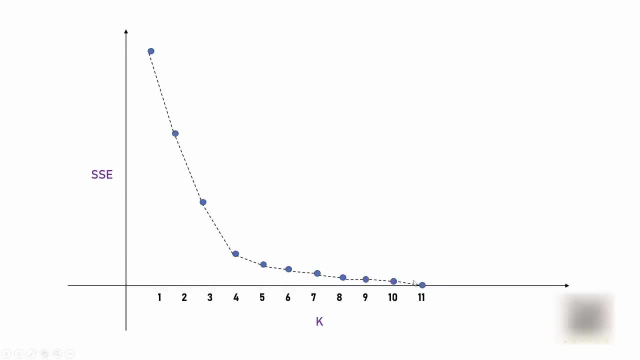 error will become 0. okay, so error will keep on reducing and the general guideline is to find out an elbow. so the elbow is on this chart. this point is short of like an elbow. okay, so here is a good cluster number. okay. so, for example, for whatever the data set, this chart is representing: 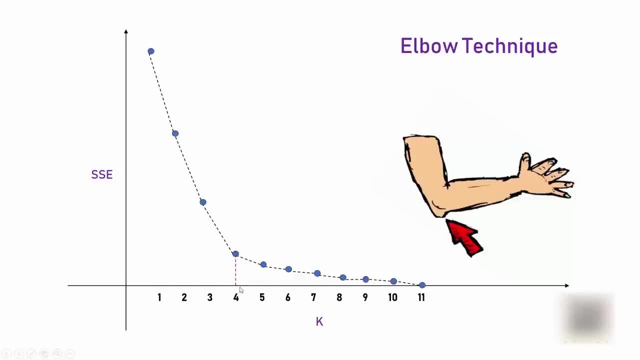 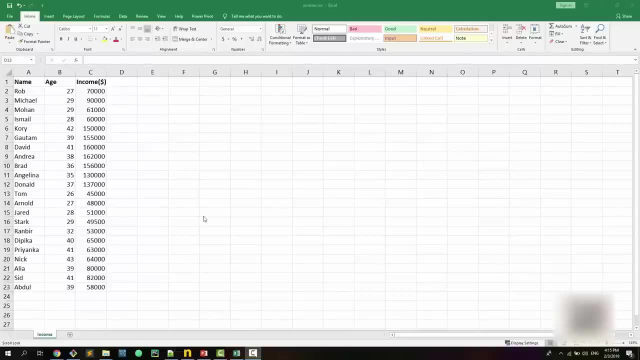 a. a good K number would be 4, all right. so that was an elbow technique. let's get into Python coding now, all right. so the problem we are going to solve today is cluster this particular data set where you have age and income of different people. now, by clustering these data points into various groups, what you're 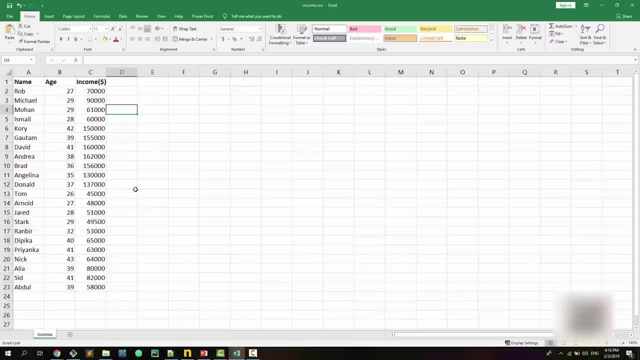 trying to find out is some characteristics of these groups. maybe the group belongs to a particular region in US where the salaries are higher, or or the salaries are lower, or maybe that, though, that group belongs to a certain profession where the salaries are higher versus less. okay, so you try to identify some. 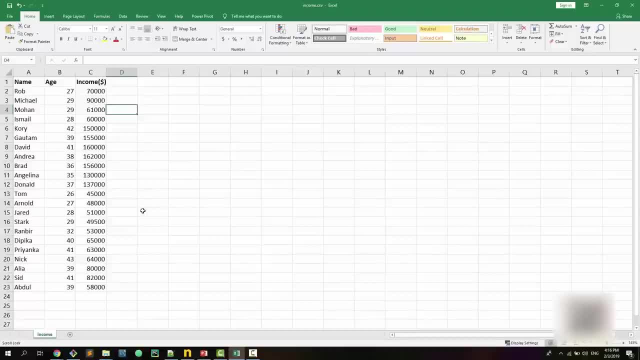 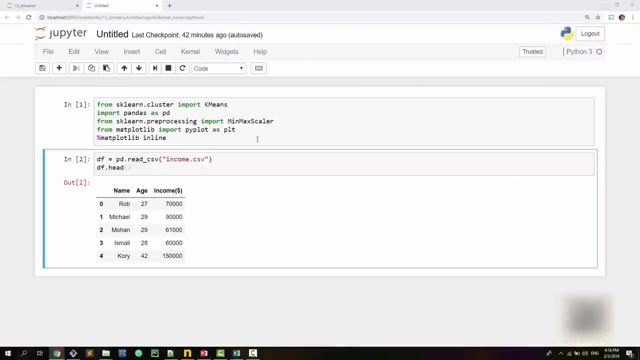 characteristics of these groups. so right now we have just name, age and income and first thing I'm going to do is import that data set into pandas data set and data frame. so you here, you can see that I imported essential libraries and then I have my data frame. 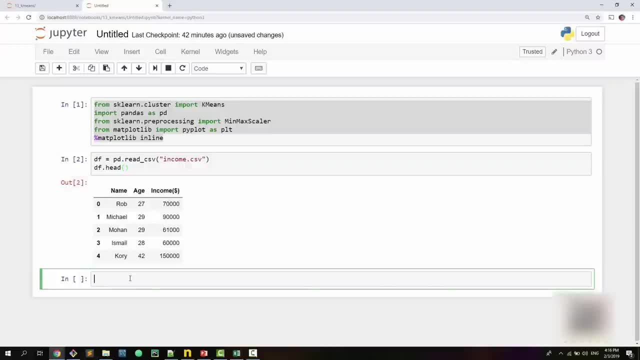 ready with that and since the data set is simple enough, I will first try to plot it on a scatter plot. okay, so when you plot it on a scattered plot, of course I don't want to include name, I just want to plot the age against the income. so df, dot, age, df. 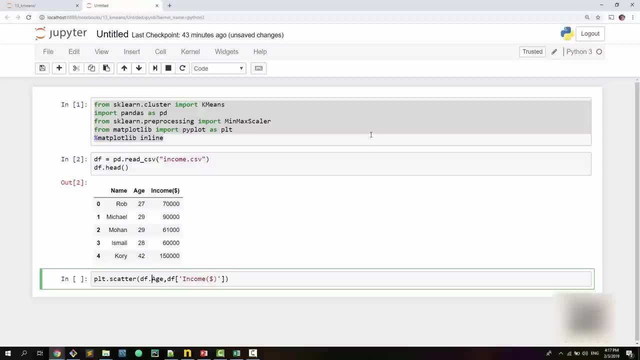 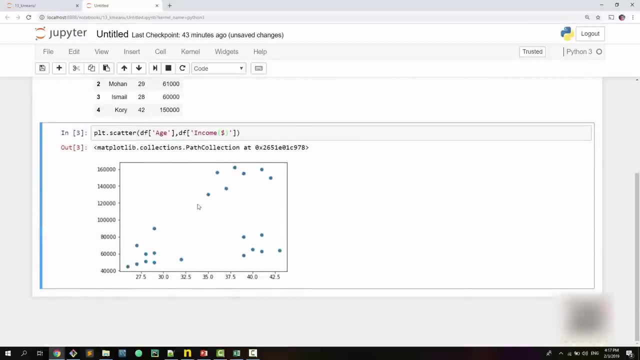 income in dollar. I'll just use the same convention. you can use dot also, but since there is a bracket here, I will use the same convention. okay, when you plot this on scatter chart, you can kind of see three clusters: one, two and three. so for this particular case, choosing K is pretty straightforward, so I will. 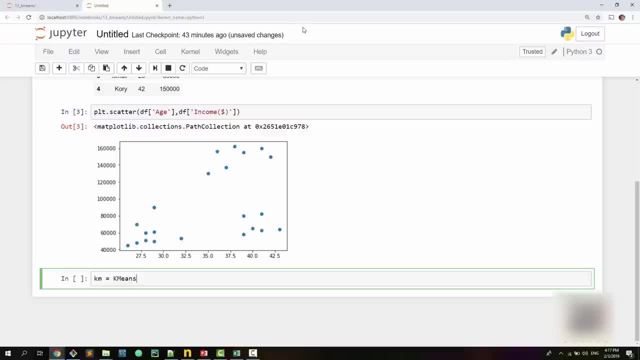 use key means. so key means is something we imported here. okay, and of course you need to specify your K, which is an underscore clusters. and, by the way, in Jupyter notebook when you type something and when you hit tab, it will auto complete. okay, so it creates this key means object for you and it has. 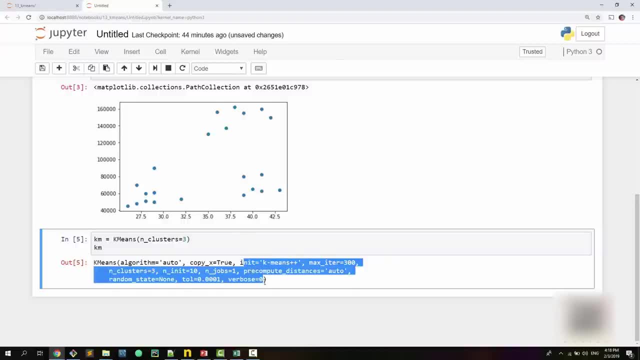 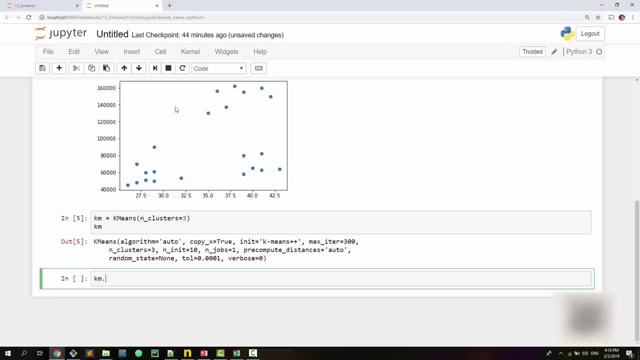 all these default parameters. you can tweak all these parameters later, but I'm just trusting on the default parameters. the second step is fit and predict. so in previous supervised learning algorithms we used to do fit and then calculate the score. here I'm just directly doing fit and predict. so fit and predict what, okay? 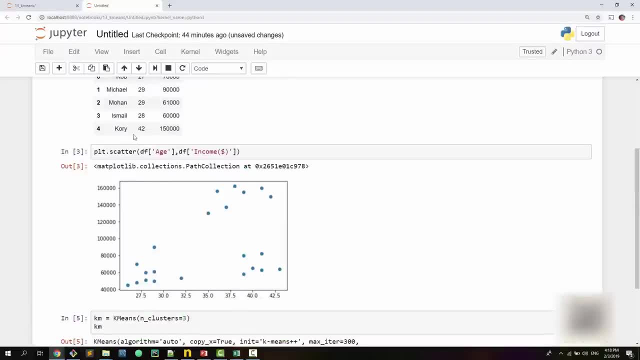 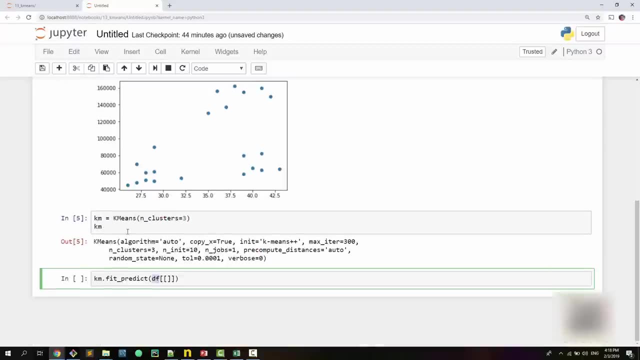 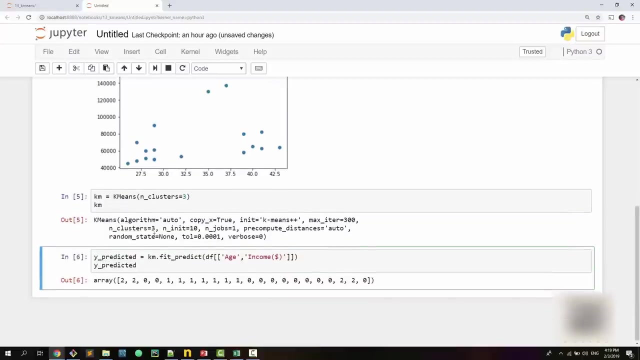 fit and predict the data frame, excluding the name column, because name column is string and it's not gonna be useful in our numeric computation, so I want to ignore it. all right, so you do fit and predict, and what you get back is why predicted. so now, what this statement did is it ran k-means algorithm on age and 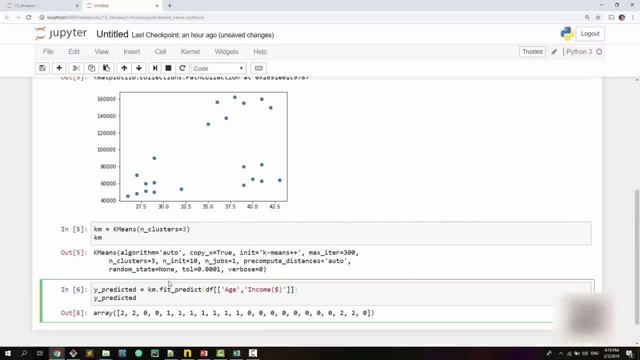 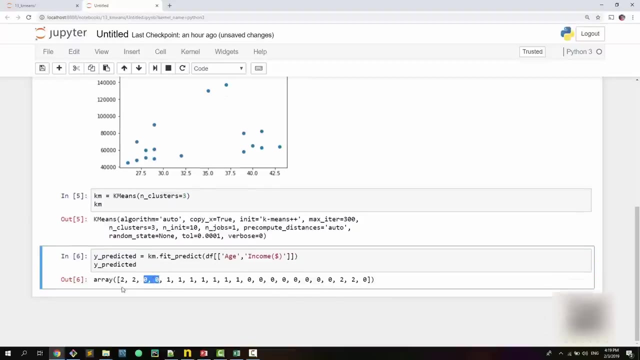 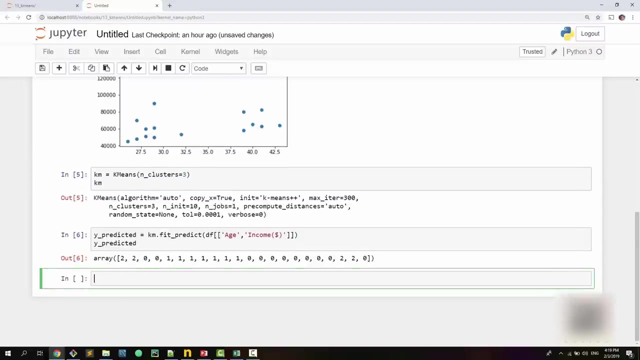 income, which is this scatterplot, and it computed the cluster as per our criteria, where we told algorithm to identify three clusters somehow. okay, and it did it. it just assigned them different labels. so you can see three clusters: zero, one and two. now, visualizing this array is not very, very much fun, so what we want to do is we: 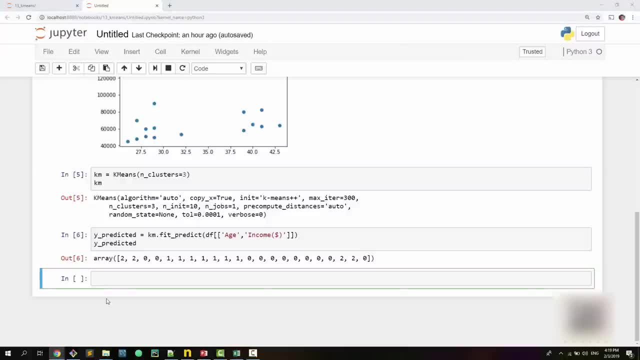 want to plot it again on on a scatterplot so that we can see what kind of clustering result did it produced. okay, so I am in my data frame. I am going to append this particular column so that my data frame looks like this: so now this is little better where I can see these two guys belong to same group. 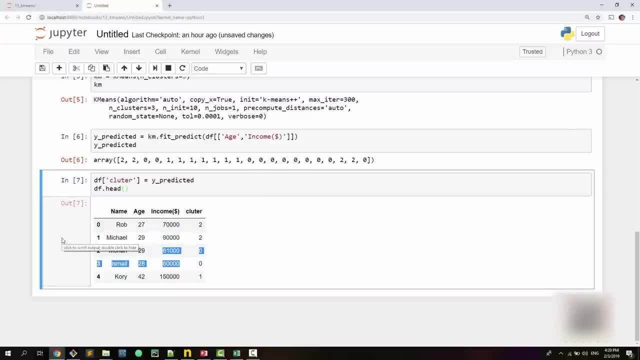 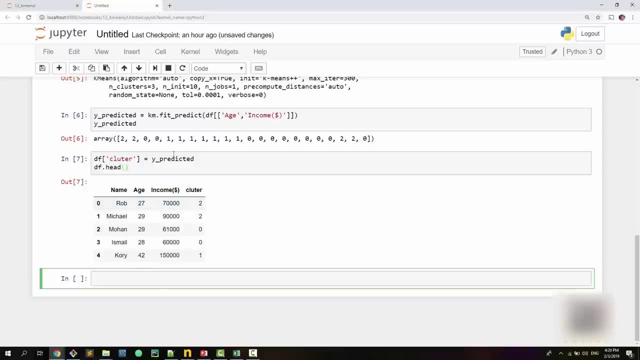 these two belong to the same group, these two belong to the same group, these two belong to same group, and so on, but it is still not as good as scatterplot, okay, so let's do this plot dot scatterplot all right. now. what we need to do is we need to. 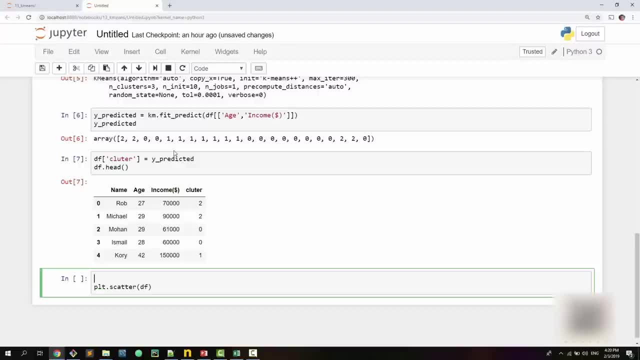 separate these three clusters into three different data frames. so let me do that. df1 is equal to df. df, dot cluster cluster is equal to zero. okay, so what this is doing is it's returning all the rows from data frame where cluster is zero, and the second one will be this and the third one will be: 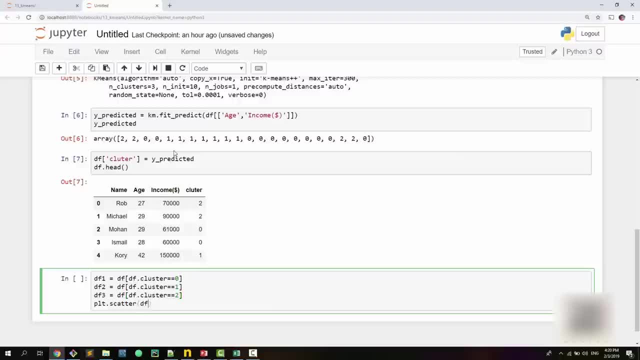 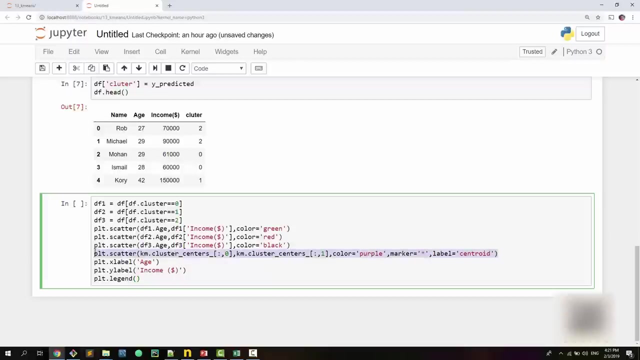 this. so now we have three different data frames, each belonging to one cluster, and i want to plot these three data frames onto, uh, one scatter plot. okay, now, just to save some time, let me just copy paste the code here. okay, i will come at this little later, but see three different data frames and we are plotting these. 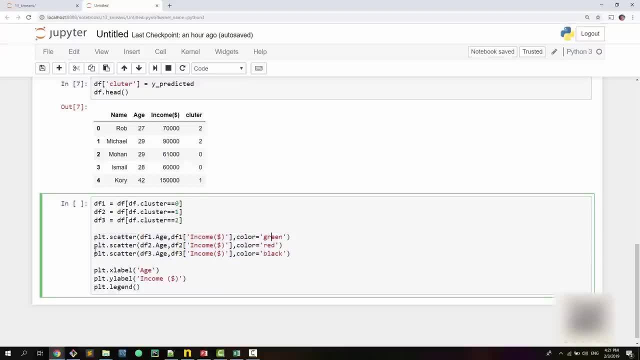 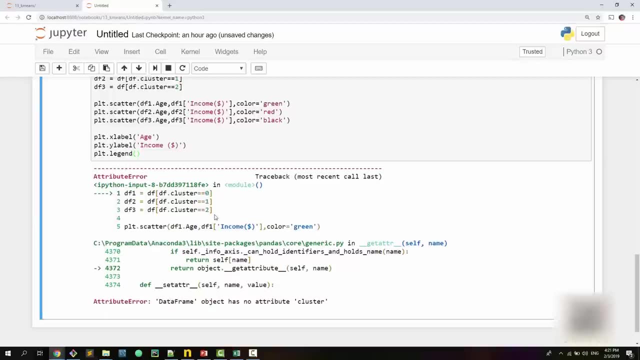 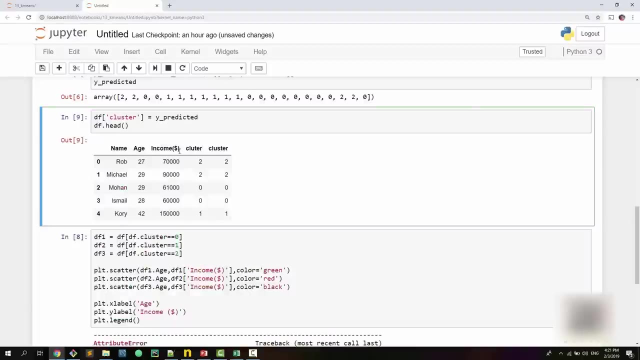 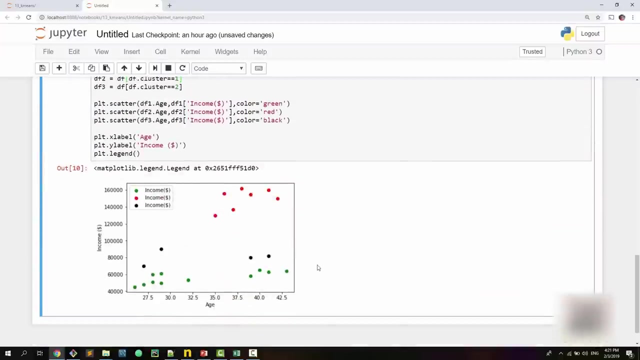 uh, data frames into different color. okay, so cluster zero is green, then red and black. let's see how that looks. okay, so df. oh, i'm made a mistake here. i had a typo. good, all right, so i see, uh, scatter plot here, but there is little problem, so this: 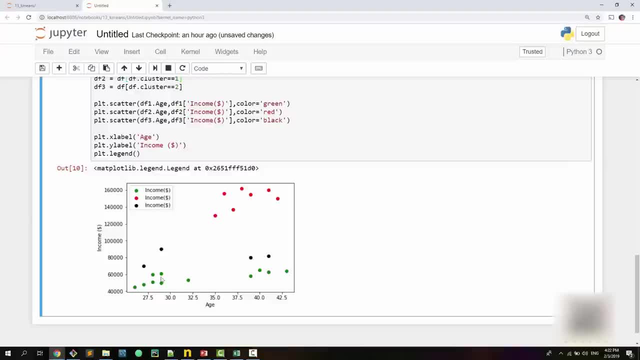 red cluster looks okay, but there is a problem with these two clusters. you know they are not grouped correctly. so this problem happened because our scaling is not right. our y-axis is scaled, uh, from, let's say, 40 000 to 160 000, and the range of x-axis is pretty narrow, so it's like hardly 20. 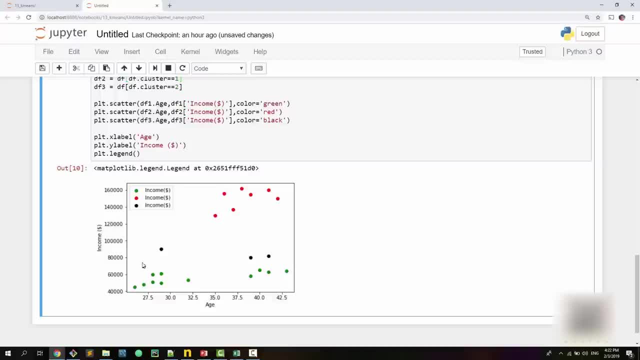 versus here is 120 000. so when you don't scale your features properly, properly, you might get into this problem. that's why we need to do some pre-processing and use min max scalar, uh, to scale these two features, and then only we can run our algorithm. all right. 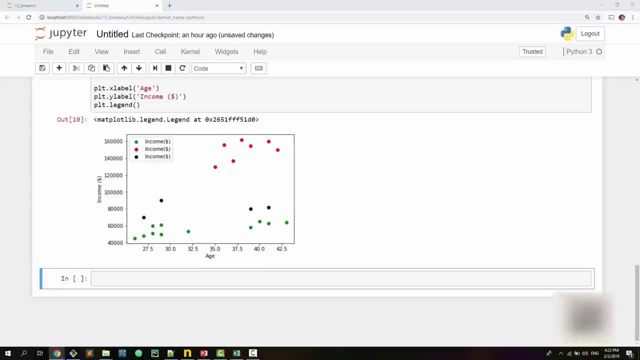 so we are going to use min max scalar. so the way you do it is, you will say: scalar is min max scalar, and this is something, if you already noticed, we imported here. okay, all right, so scalar is this and scalar dot fit df. so now i want to fit first the 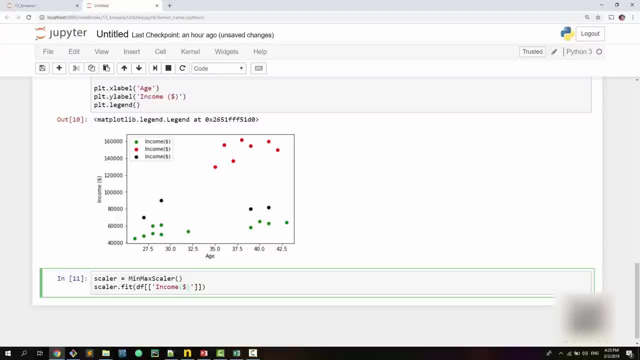 income. all right, so my scalar- min max scalar- will try to uh make the scale zero to one. so after i'm done with my scaling, i will have a scale of zero to one on y as well as x-axis. all right, so, df, let me just copy paste this guy here. 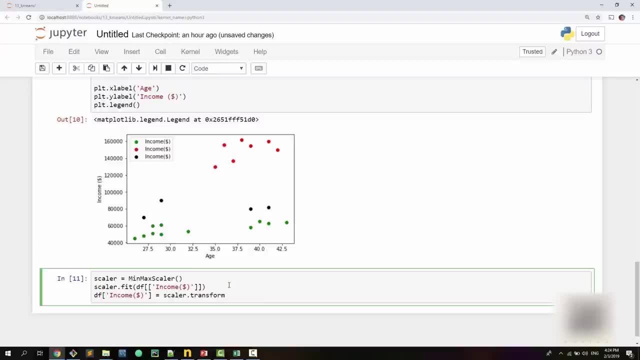 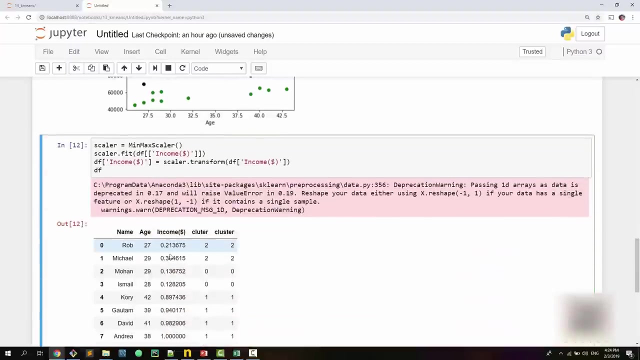 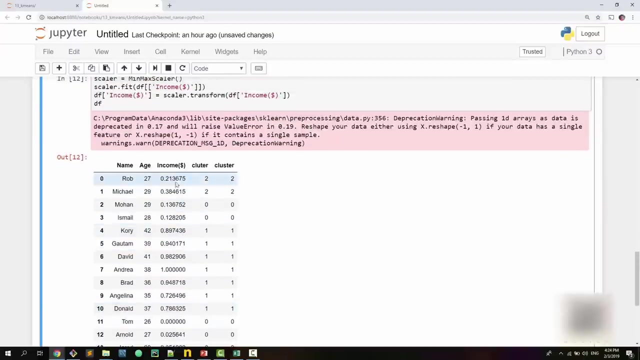 is equal to scalar dot transform. okay, so now scalar will um scale the income feature. all right, so df this. okay, let's see how that did it, so you can see that the income is, uh, scale, right, it's like see 0.21, 0.38 and so on. so it is in a 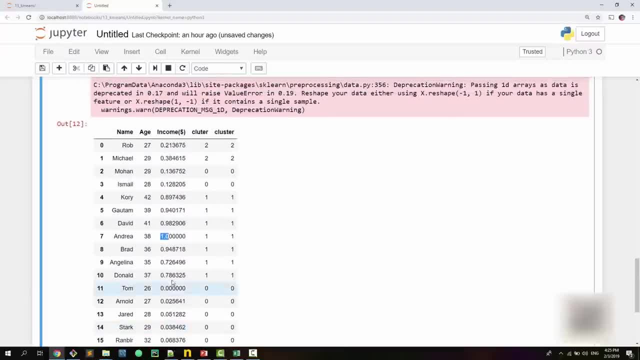 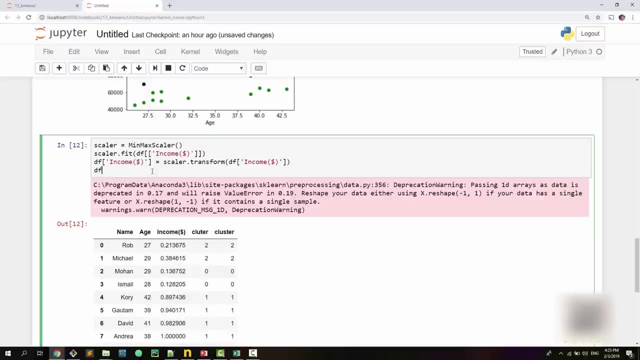 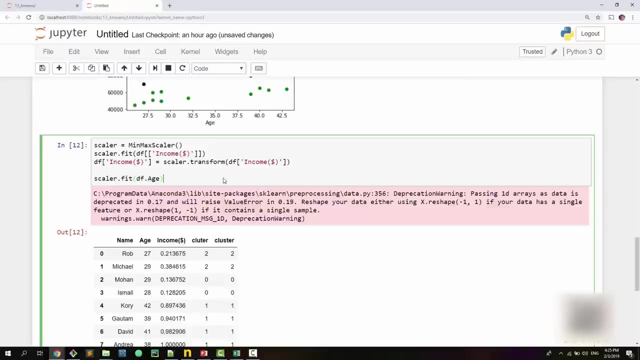 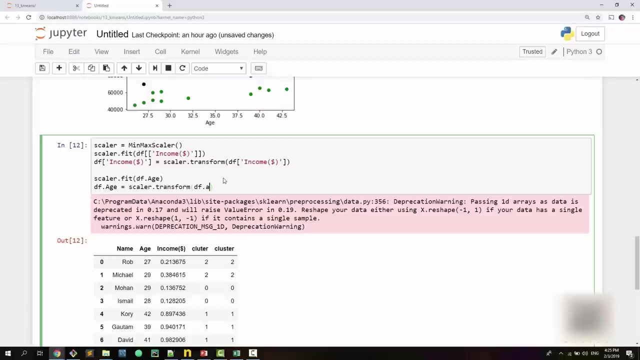 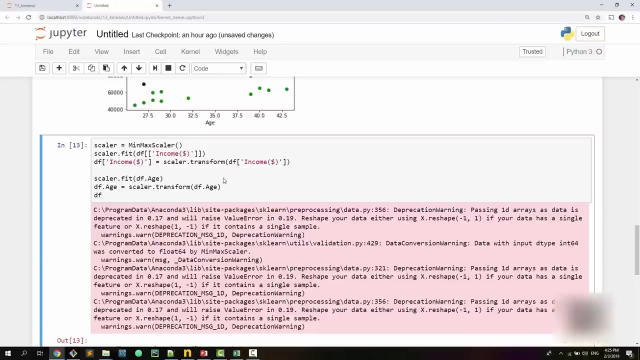 range of one to zero. you will not see any value outside zero to one range. we want to do the same thing for our age also. okay, so let's do that. scalar dot fit df dot age. df dot age is equal to 0.28. scalar dot transform df dot age and then we print our df. 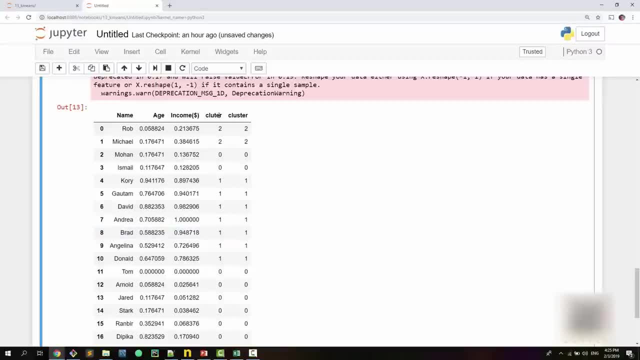 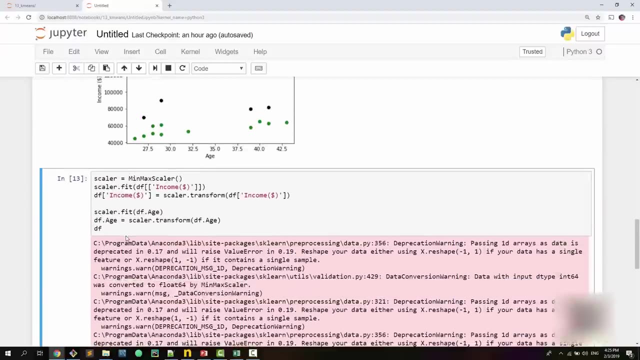 and you can see the age is also scaled. okay, i have this extra column because i made a mistake previously, but you can ignore that. you can ignore cluster also. so we have age and income features properly scaled now. okay, and even if you plot these onto scatter plot, they will look structure wise. at least they will look like this: 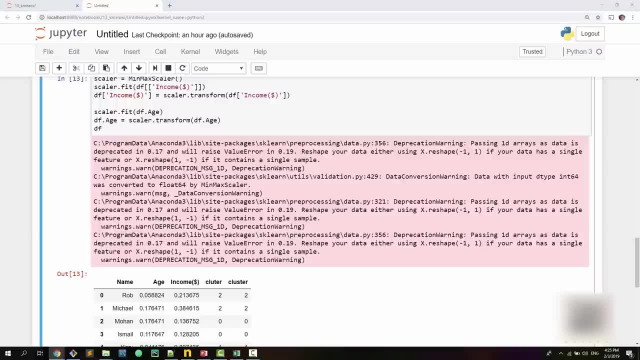 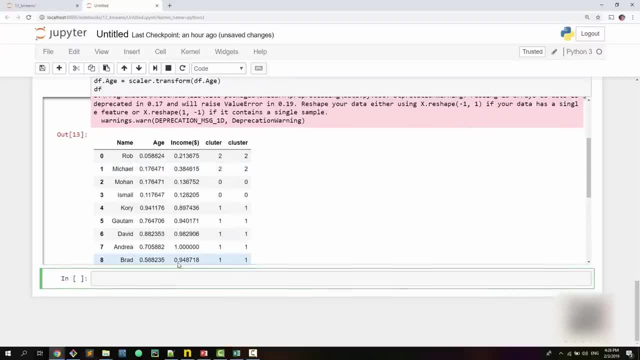 okay, all right. so the next step is to use k-means algorithm once again- uh, to train our scale data set. this is gonna be fun. now let's see what scaling can give us. and, as usual, y-axis is equal to zero. this is the value of y-axis, and we can use the value of cn to back it up to the value of t, which is really important, and we're not going to kidding you, remember? we don't want to use cn for that anymore. we're going to simply use the value of e and we're not going to focus the value of t on the cn. so we're going to focus the value of t on the t. 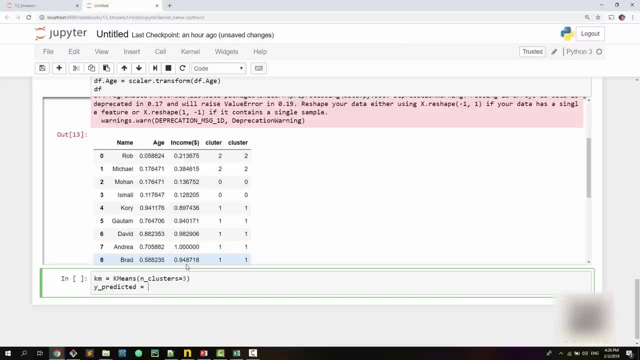 and we're going to focus the value of c if we want to use our e instead of e, and we're going to focus the value of e to the cn. so this is not something that we'll use here. y predicted is equal to km dot fit and predict. so again, I started with three. 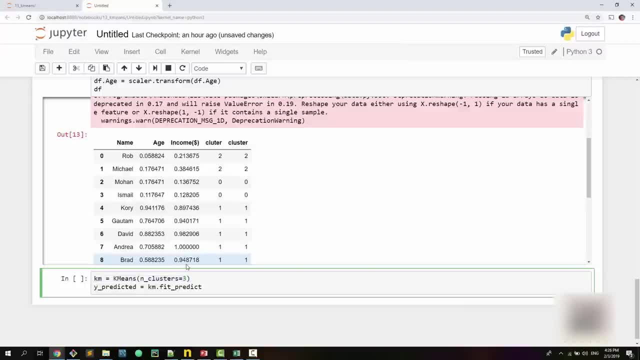 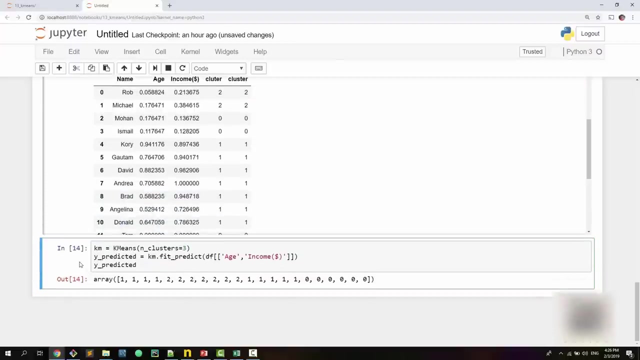 clusters and I'm using- I'm just fitting my scale data- age, income, all right, and let's see my y predicted. so it predicted some values which yet don't know how good they are, so I will just do: cluster is equal to Y predicted. I would also 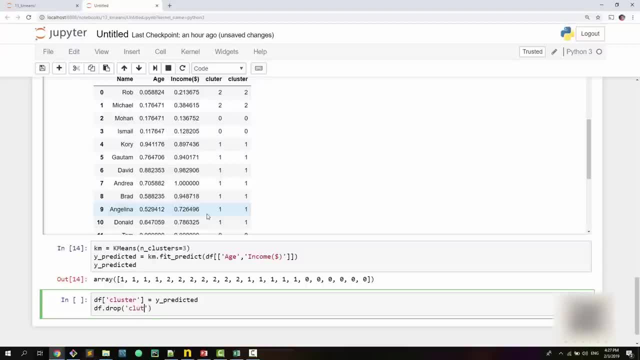 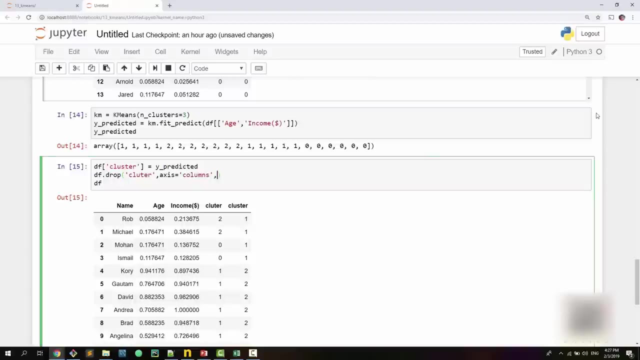 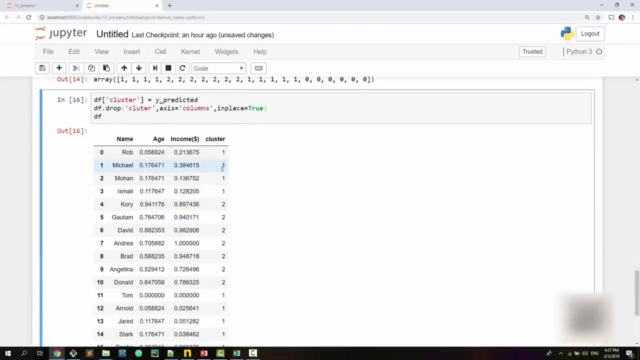 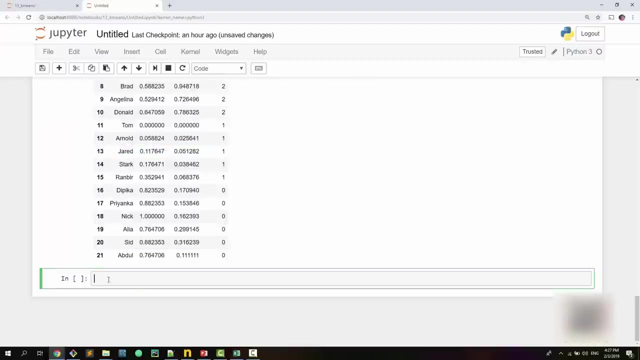 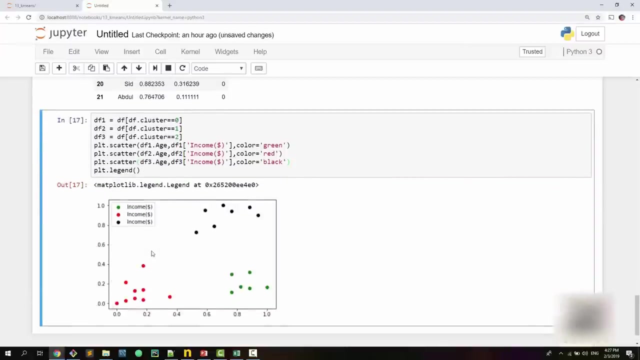 just drop the column that we typo'd. and then let's look at D, f, okay in places. in place is equal to true, okay. so now this is my new clustering result. let's plot this on to our scatter plot. i'm just going to remove this for now. now you can see that i have a pretty good cluster, see black. 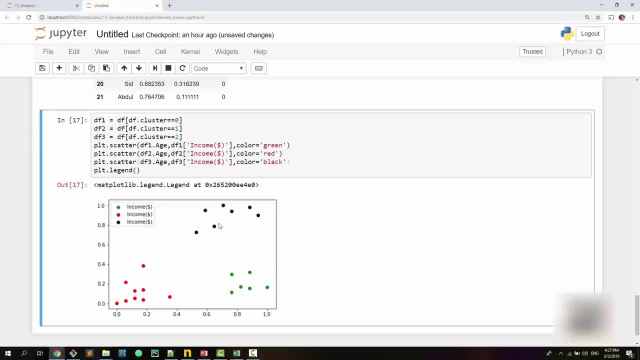 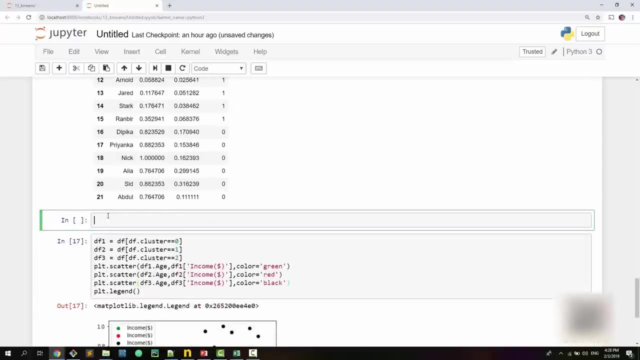 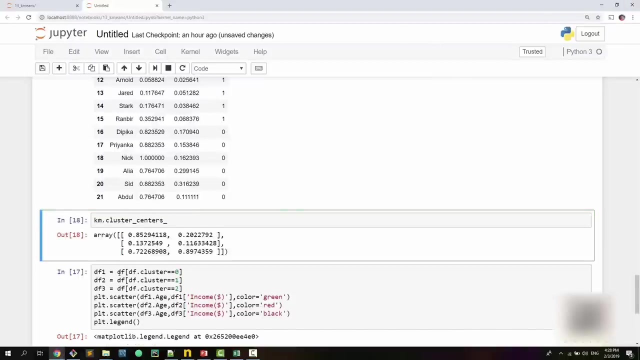 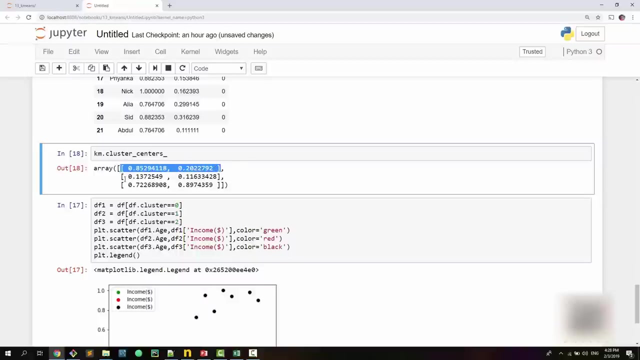 green and red. they look very nicely formed. one of the things we studied in our theory section was centroids. so if you look at km, which is your train or k-means model, that has a variable called cluster centers and these centers are basically your centroids. okay, so this is x, this is y, so this is the first centroid of your first cluster. 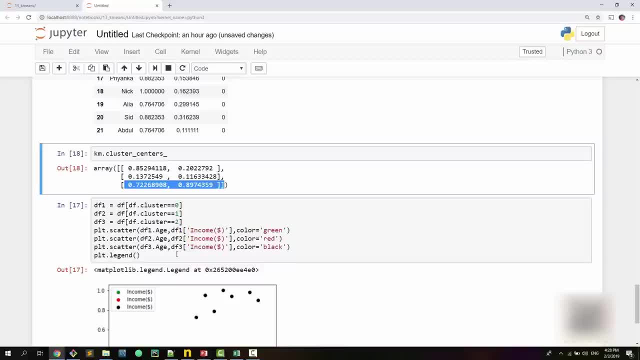 second centroid and third centroid. and if you can plot this into a scatter plot, uh, it can give a nice visualization to us, right? so pld, dot scatter, okay. so first let's plot x axis. okay, so, x axis for this will be. it will be what? okay, so. 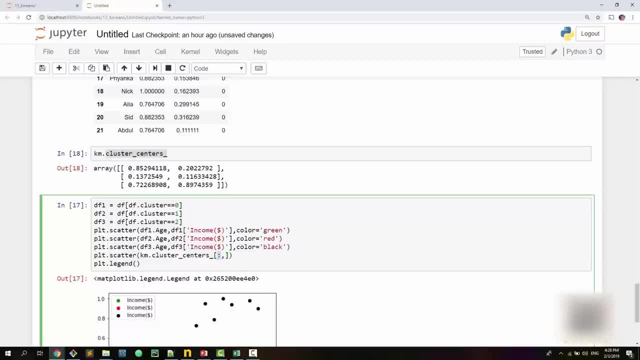 using this syntax you can say: i want to go through all the rows, which is three rows here, and then the zero min first column, which is this okay, and your y is your first column. and just to differentiate them with regular data points, i will use some spatial marker and color. 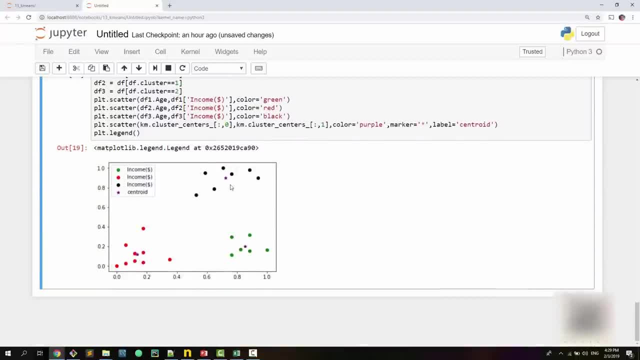 so you can see that these are the centers of my clusters. all right, let's look into now elbow plot method. see, this is my cluster and this is the center of my cluster. when we plot this, we should see that these are the centers of the clusters. all right, let's look into now elbow plot method, see. 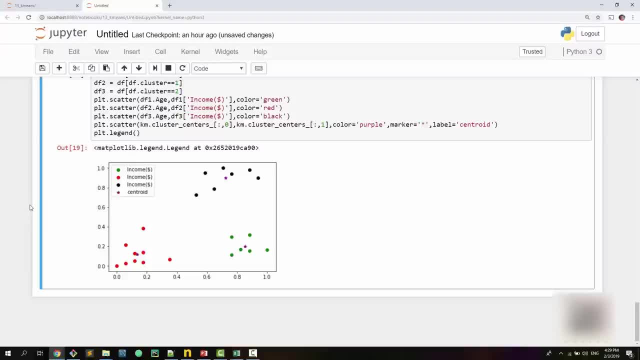 data sort was simple, but when you're trying to solve a real-life problem, you will come across data set which will have like 20 features. it will be hard to plot it on a scatter plot and it will just get messy and you'll be like what? 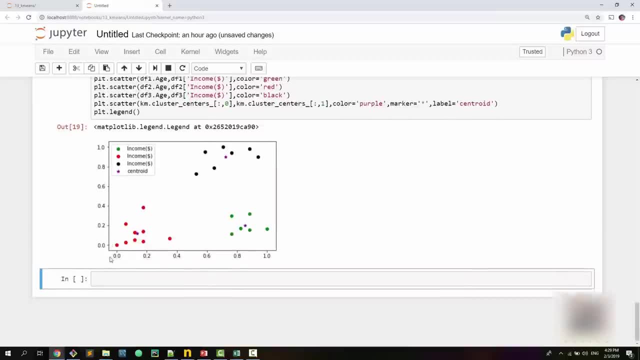 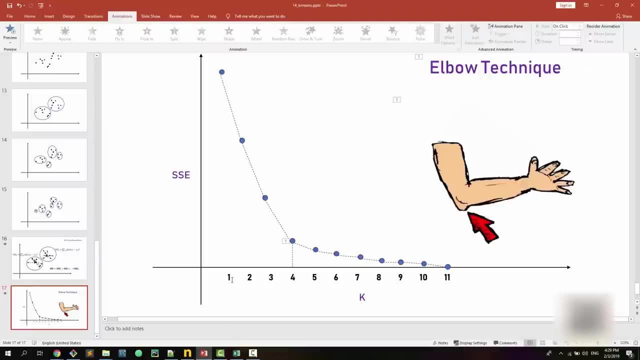 do I do now? well, you use your elbow plot method. so in elbow plot, as we saw in theory, we go through number of case. okay, so let's say we'll go from K equal to 1 to 10 in our case, okay, and then we try to calculate SSC, which is sum of 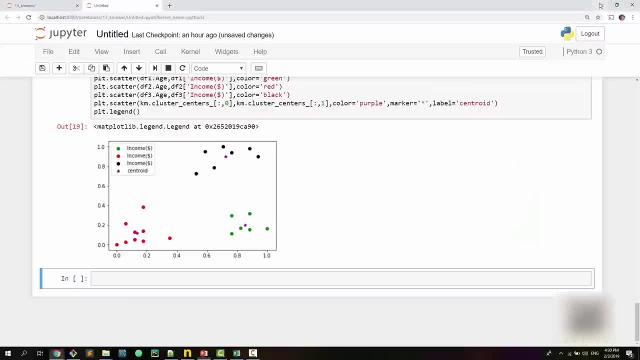 squared error and then plot them and try to find this elbow. so let's define our key range. let's say I want to do 1 to 10, this will be 1 to 9, but whatever. okay. and then sum of squared error is an array. so for K is equal to 1, you'll find. 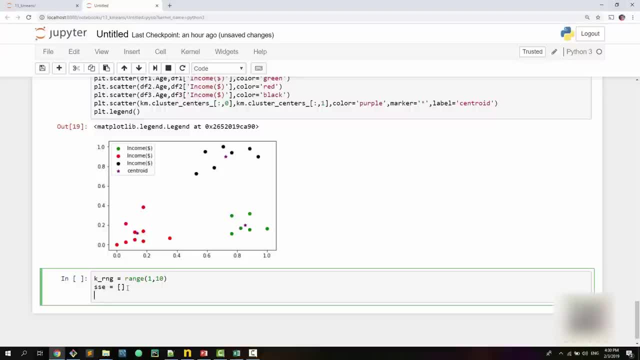 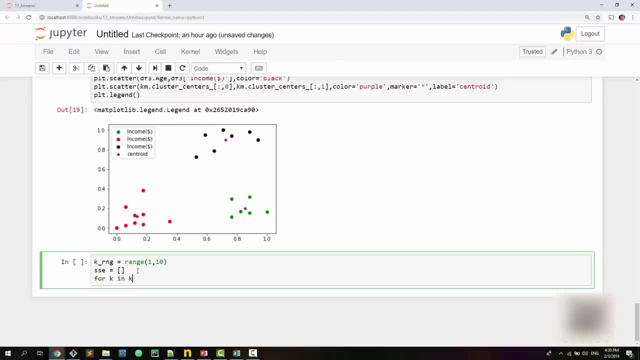 Figure scores to table in an energy table. to table one and two in the table. we need to do matter for a sse k equal to 2, you will find sse. you will store all of that into this array and then use matplotlib to plot the result. okay, so for k in k range. so i'm just going through. 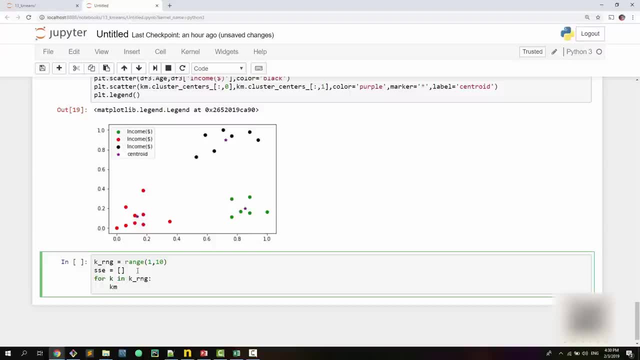 1 to 9 and then each iteration. i create a new model with clusters equal to k. okay, and then i call fit. okay, and what? what do i try to fit? okay, i try to fit my data frame, but i use this syntax because my data frame has name column. i don't want to use name column. 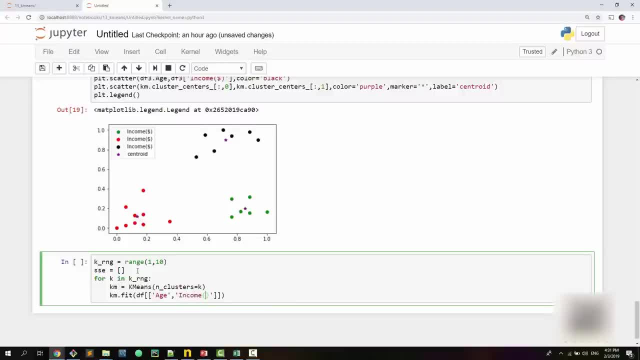 all right, you'll be like what the heck this guy is doing all the time using this crazy syntax, but that's to avoid name. if you want, you can just create a new data frame, just drop name column, name column and then make sure that you don't have to do anything like that. okay, and if you? 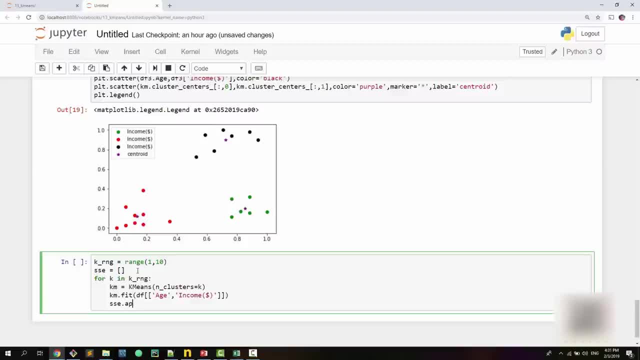 don't want to make it. you can just create a new product and then you can just create a new data from. that is fine too, and all right. so now, what is my sum of square error? how do i get that? when you call kmfit, after that on your k means there is a parameter called inertia. 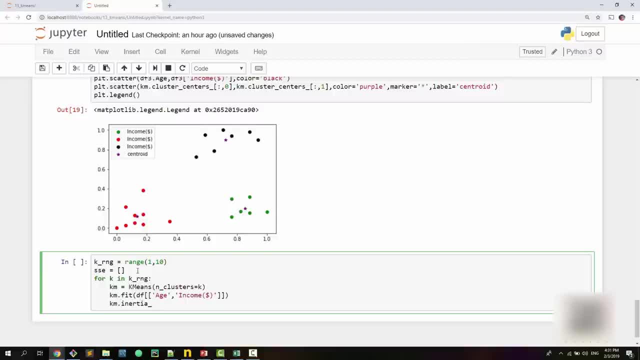 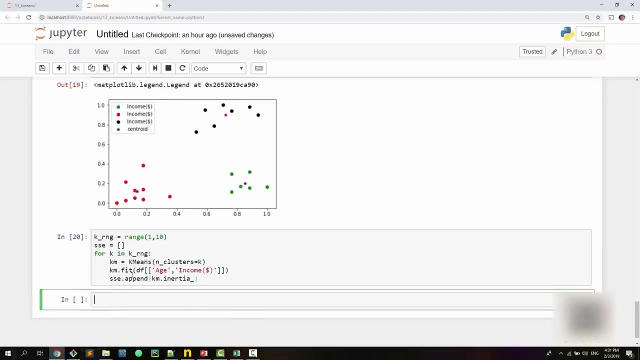 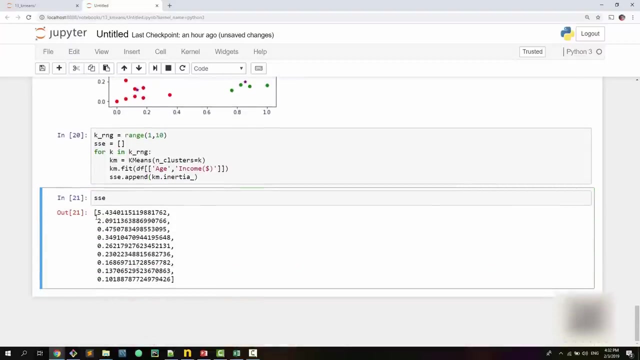 that will give you the sum of square error and that error. we want to just append it to our array that we have. all right, that was pretty fast because our data set is very small. okay, let's see what is sse. so sse: you can see that sum of square error was very high initially. 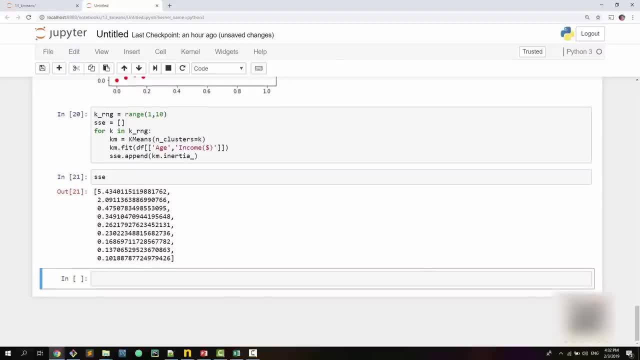 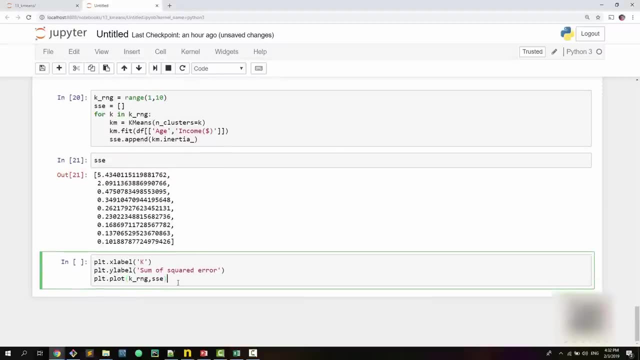 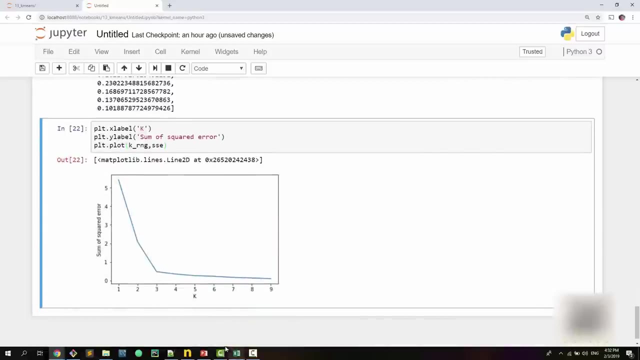 then it kept on reducing. and now let's plot this guy into nice chart. so, let's plot this guy into nice chart. so let's plot this guy into nice chart. okay, when you do that, you get our elbow plot. remember elbow plot, elbow, all right, where is? 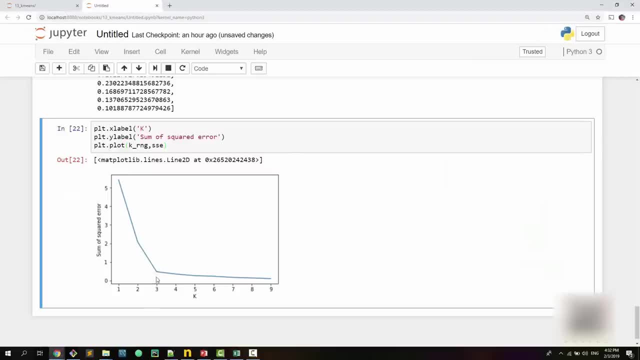 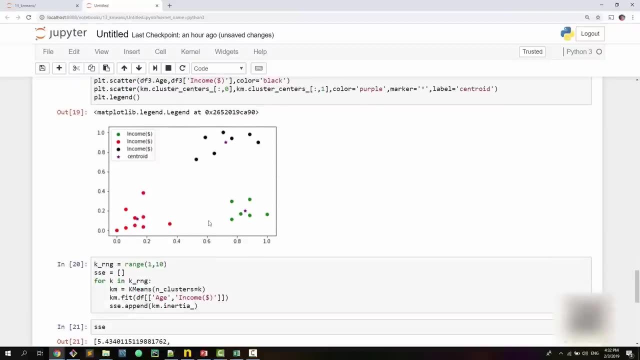 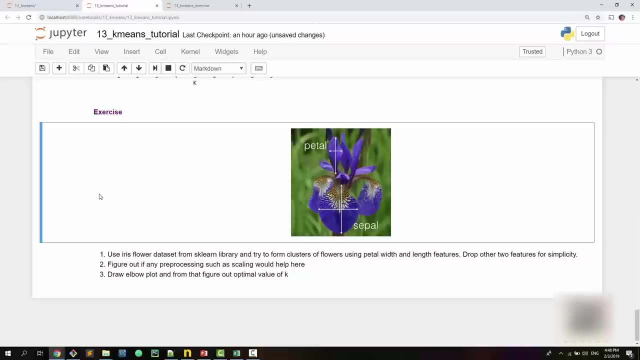 my elbow. where is my elbow? okay, here is my elbow. you can see that k is equal to three for my elbow, and that's what happened. see, i have three clusters for exercise. we are going to use our iris flower data set from sk learn library and what you have to do is use 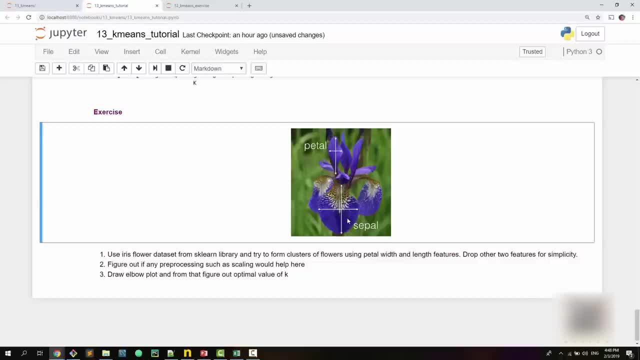 your patel length and width features. just drop sapl length and width because it's it makes your clustering a little bit difficult, so just drop these two features for simplicity. now that data set has a class label in the target variable, but you should just ignore it. okay, you can.